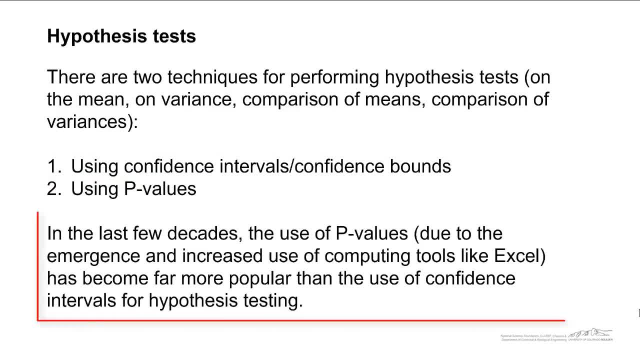 which entails using p-values. In the last few decades, the use of p-values, due to the emergence and increased use of computing tools like Excel, has become far more popular than the use of confidence intervals for hypothesis testing. The techniques in this screencast actually aren't. 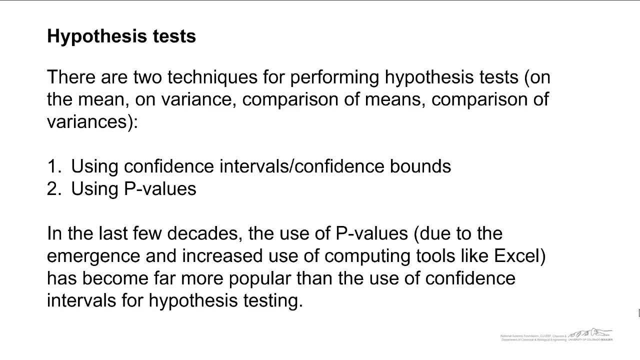 used as frequently as p-values in hypothesis testing. The techniques in this screencast actually aren't used as frequently as p-values in hypothesis testing. The techniques in this screencast actually aren't used as frequently as p-values in hypothesis testing, So just keep that in. 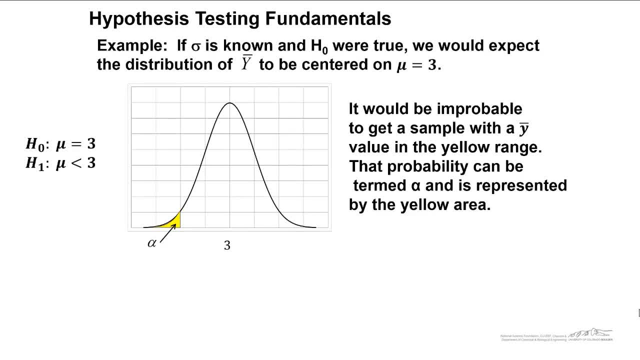 It looks like you can see how lower version alpha is lower than alpha. It's the same. Keep that in mind. If we plotted our sampling distribution, our random variable is y. so if we plotted y-bar, if it were centered on mu equals three, then this is what the sampling 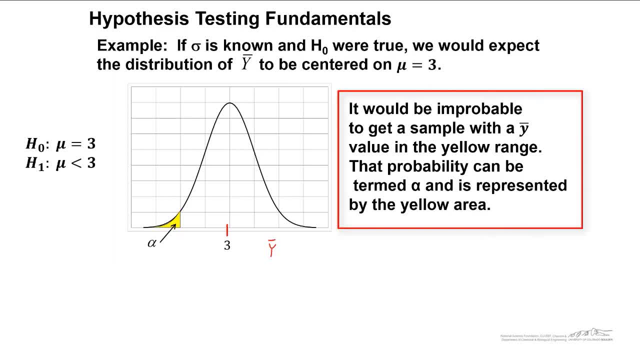 distribution would look like. It would be improbable to get a sample with the y-bar value in the yellow range and we call that alpha, the risk level, For example. alpha could be 0.05.. If the true mean of ride time is three, it would be rare that we get an average of ride times. 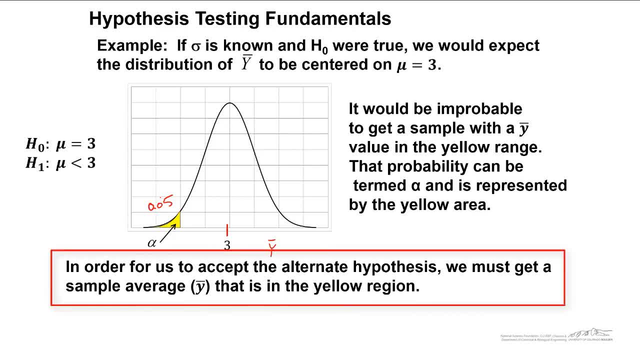 somewhere between zero and a half. Baohtman experiment: If true, mean of ride time is somewhere down in this yellow region, In order for us to accept the alternate hypothesis we have to get a sample average that is down in the yellow region. And if we were to get 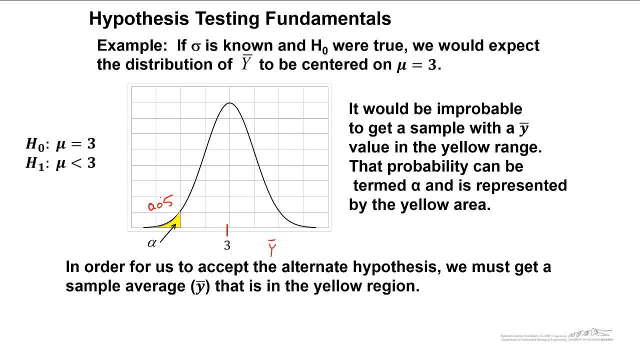 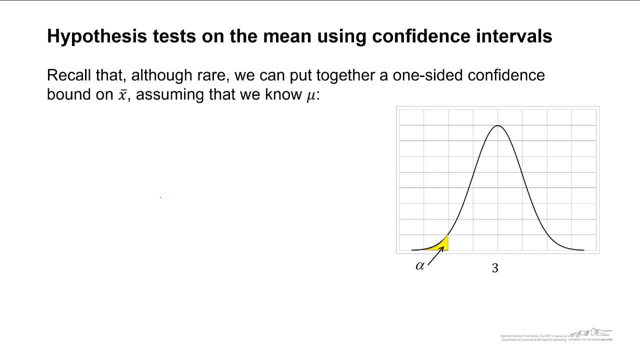 a sample average down in that region, we would accept the alternate hypothesis and reject the null hypothesis. So let's talk about how we can use confidence intervals or confidence bounds. Confidence bounds are one-sided confidence intervals. Although one-sided confidence intervals or bounds are rare, we can put together a confidence bound on x-bar- the sample average. 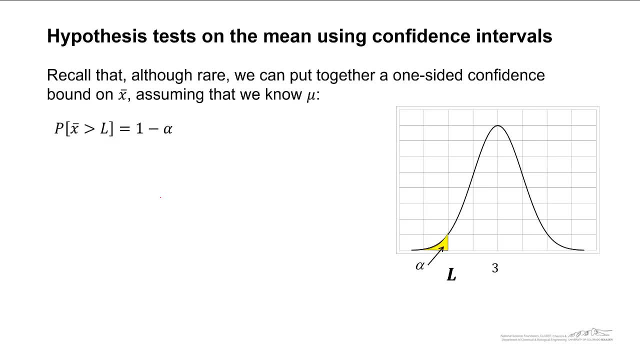 assuming that we know mu Recall that the probability that the sample average is going to be greater than L again here on the right we have a sampling distribution- is equal to 1 minus alpha. If alpha were 0.05, then we would have a 95% chance of getting an average. 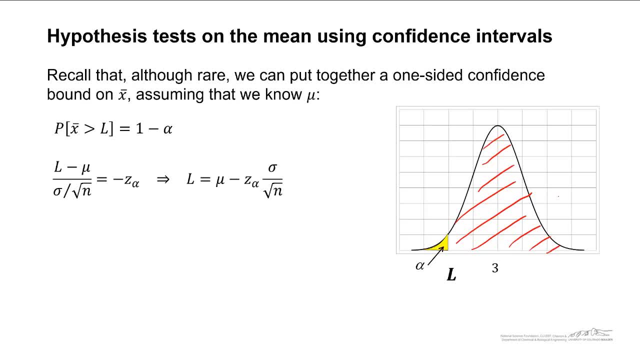 in this red shaded region. We can convert L to a 0.05.. We can convert L to a standard normal variable negative z alpha, That is negative of the z value containing alpha percent to the right. And if we solve for L, the lower limit here. 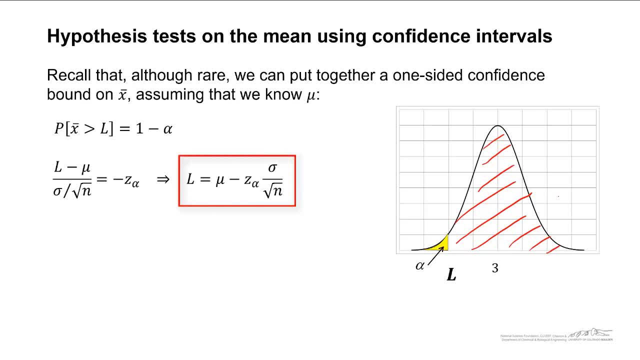 for x-bar. we get that that is equal to mu minus z alpha times sigma divided by root n. We can rewrite the probability that x-bar is greater than L. We can substitute L into our expression and that means we have a confidence bound a 1 minus alpha percent confidence. 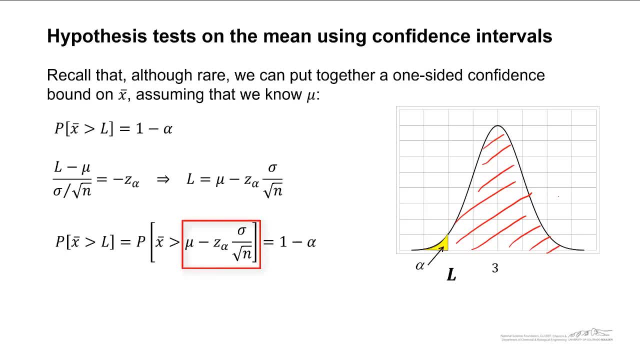 bound on x bar of mu minus z alpha times sigma over root n. So we are 95% sure, if alpha equals 0.05, that the sample average is going to be greater than mu minus z alpha times sigma divided by square root of n. If the null hypothesis is not incorrect or not false, and the true mean is mu, 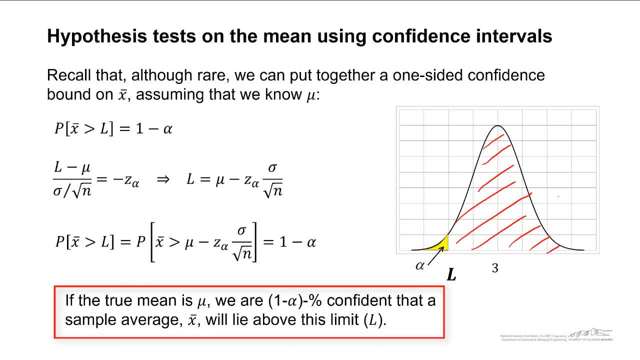 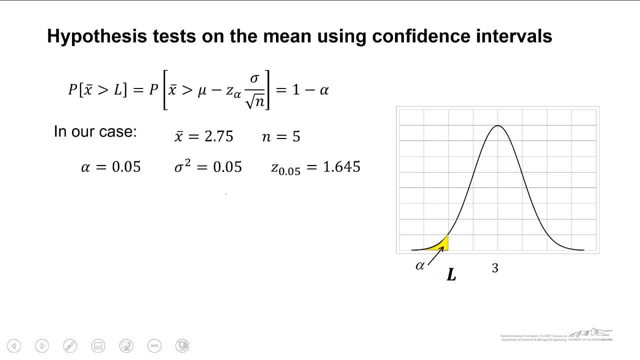 we are one minus alpha percent confident that a sample average will lie above this limit, l which we can compute here. So this is actually l In our case. we can go ahead and compute our statistics. We know that the sample average of five rides is 2.75.. We're going to use a 95%. 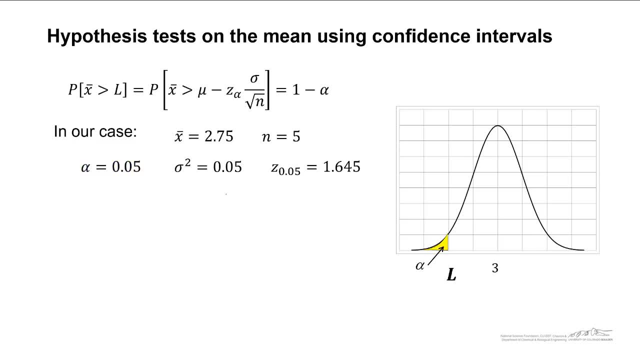 confidence interval alpha equals 0.05.. We know that the variance is 0.05 from a long history of these rides. We can compute z alpha z of 0.05 is 1.645.. And when we plug these values in, 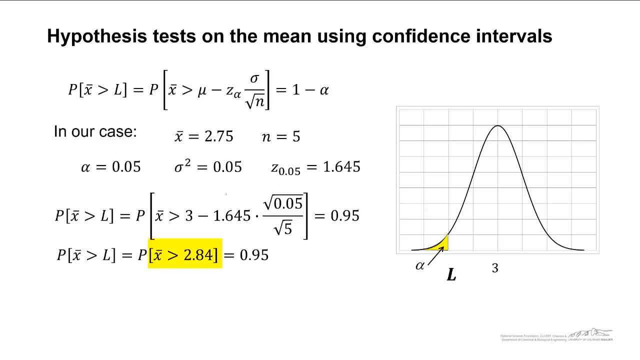 to our confidence bound above, we get that there's a 95% chance that x bar is going to be greater than 2.85.. In other words, this lower bound here that has 95% of the sampling distribution above it is 2.84.. If the true mean. 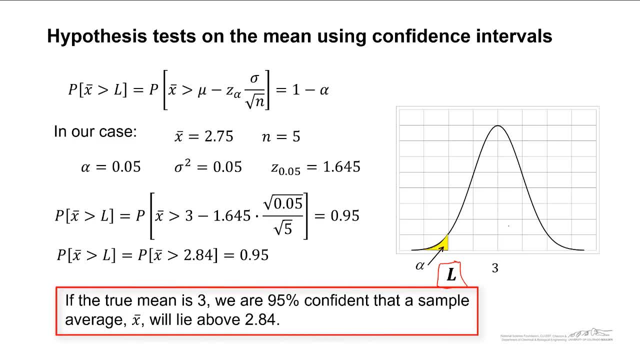 is 3, we are 95% confident that a sample average will lie above 2.84.. Consequently, obtaining a sample size n equals 5 of less than 2.84, that's down in the lower bound. here we get that the 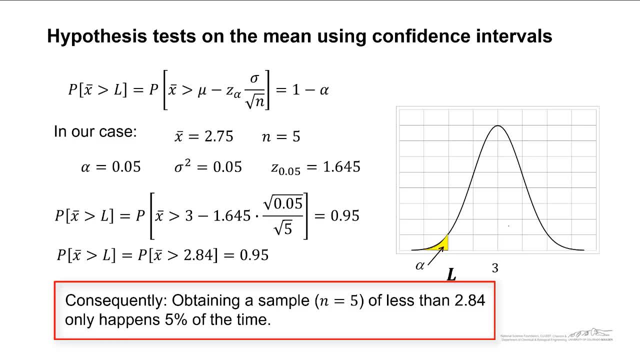 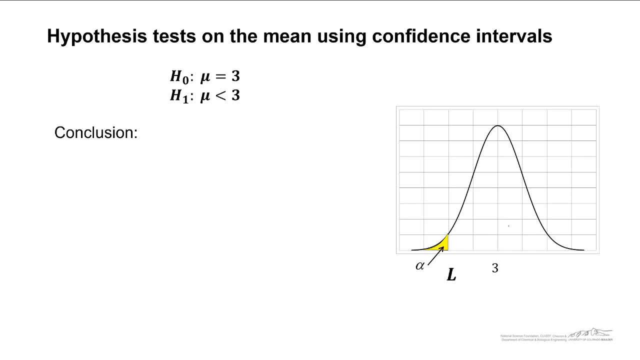 trying to explain theślę, and we're 95% sure that x bar is greater than 2.84. each waits two times more than the time is 3. And we conclude that this is rare. As a result, we accept the alternate hypothesis and. 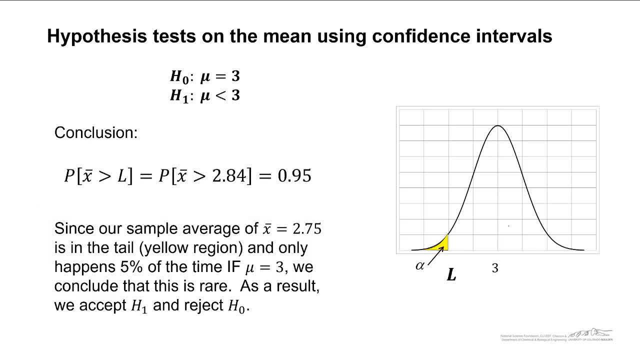 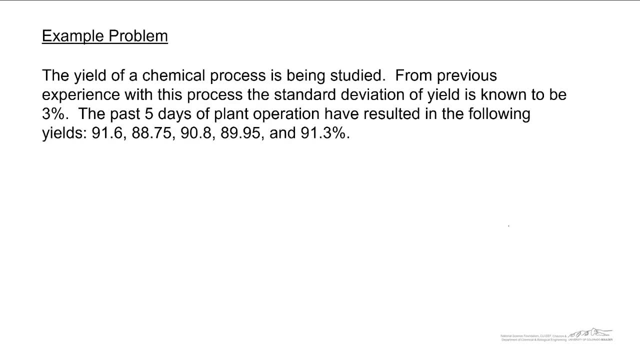 we reject the null. In other words, we can accuse Elitch Gardens of shorting us on our time on the bumper cars. Let's look at a second example: The yield of a chemical process being studied. We know from previous experience that the standard deviation is known to be 3%. The past five 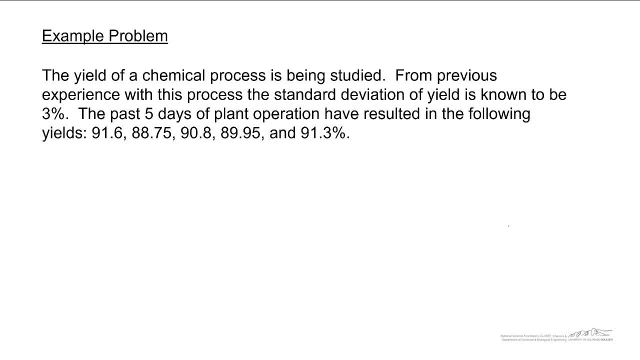 days of plant operation have resulted in the following yields: Perhaps you are a quality control engineer with the company and you just want to do routine testing to make sure that you are not varying too much from 90%. Is there evidence that the mean is significantly different? 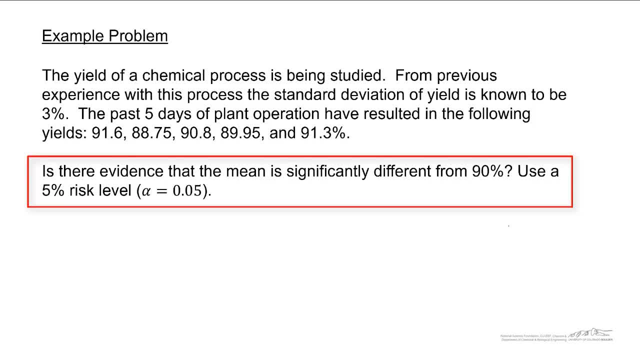 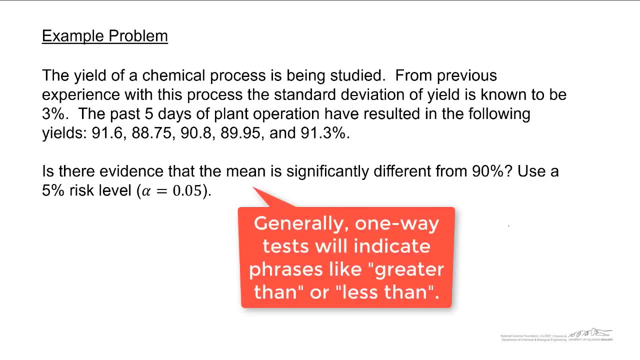 from 90%, Use a risk level of 5%. Now the problem sort of just asks: is there evidence that the mean is different from 90%? This is sort of an open-ended hypothesis test. You could be greater than 90% or you could be less than 90%, And we want to test either way. 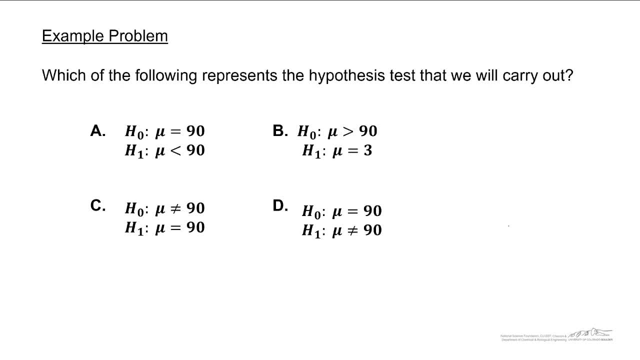 Is there evidence that we're significantly different from 90%? Which of the following represents the hypothesis tests that you should carry out? If you selected D, you are correct. The null hypothesis is: the mean is 90.. The alternate hypothesis is that the mean is. 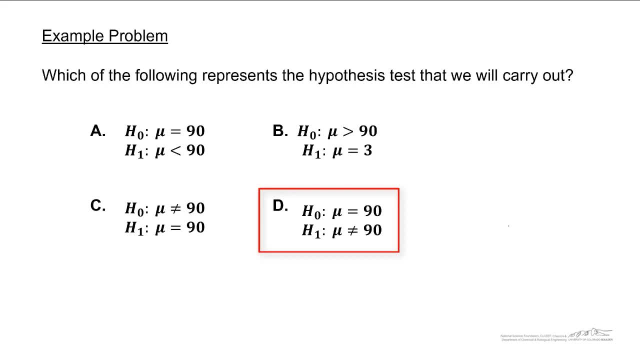 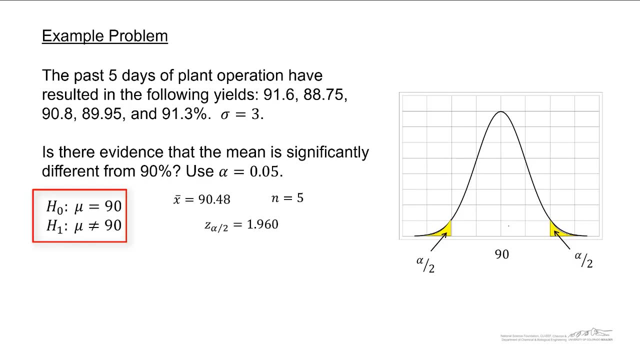 different, significantly different, from 90. That means it can be less or that means it can be greater. So we set up our hypothesis test. We're going to test the mean, We're going to test the hypothesis test. We can collect our sample statistics. n equals 5.. If I go into Excel and 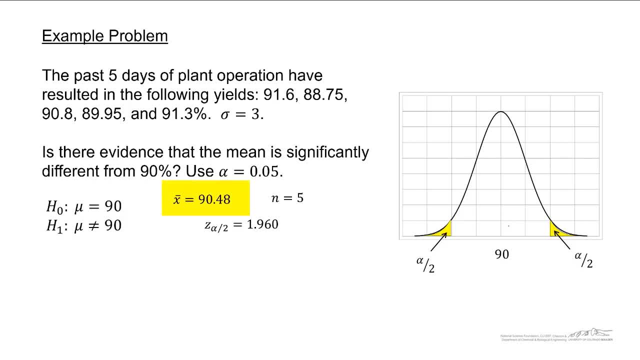 compute the average of these values, I get 90.48.. We're going to be splitting alpha into two tails because this is a two-tailed test. It's a not equal to test Z. alpha over 2 is equal to 1.960.. 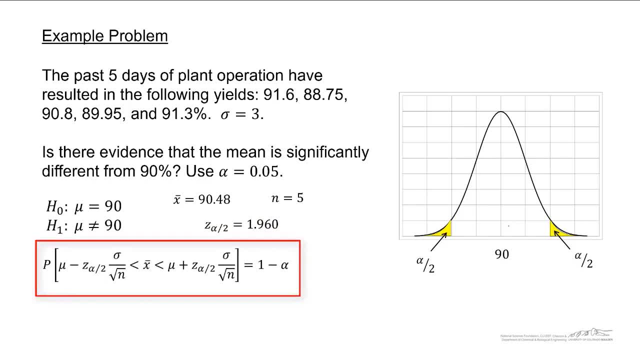 We can set up a 1 minus alpha confidence interval on this scenario. We are 1 minus alpha per cent sure that X bar lies between mu minus Z alpha over 2 times sigma over root n and mu plus Z alpha over 2 times sigma over root n. So this just goes back to the screencasts on confidence. 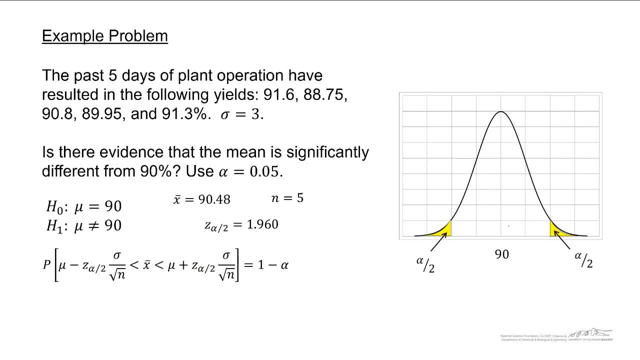 intervals. We can plug in our sample statistics and our Z alpha over 2. And when we do that, we get that there's a in our case, because alpha is 0.05, this is a 95% confidence interval.